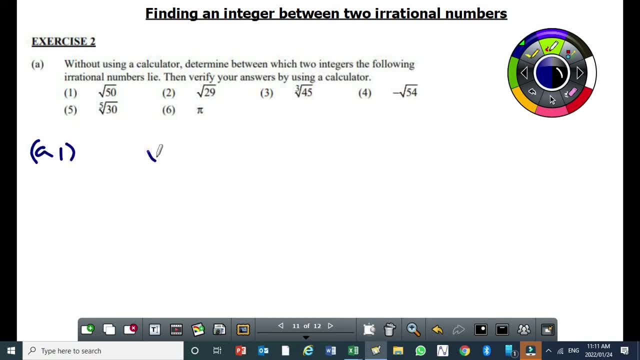 So a1 square root of 50.. I want you to pay attention carefully here. I want you to pay attention very carefully. So the question says: without using a calculator. you are not supposed to use a calculator. determine between which two integers, okay, between the following relational numbers line: then verify your answers by using your calculator. 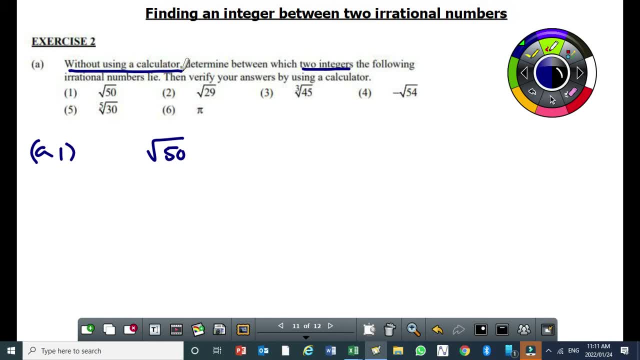 So you do the verification in the end, But you need to first do it without a. what A calculator. All right For a while, just for a few seconds, right? Okay, About the square root, Which perfect square, is close to 50 and it is also greater than 50?. 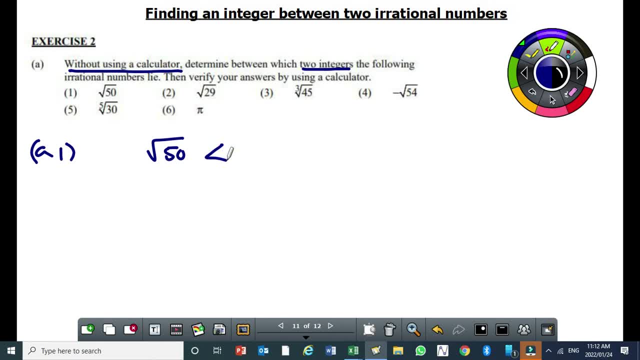 Which perfect square is greater than 50? Which perfect square is greater than 50 and it is close to 50? What? 54.. Thank you. Once we identify that, then we also have to find its square root. All right, Then, which perfect square is less than 50 but close to 50?? 49.. So we put 49 here, Right? What this means is square root of 50 is between square root of 49 and square root of what. 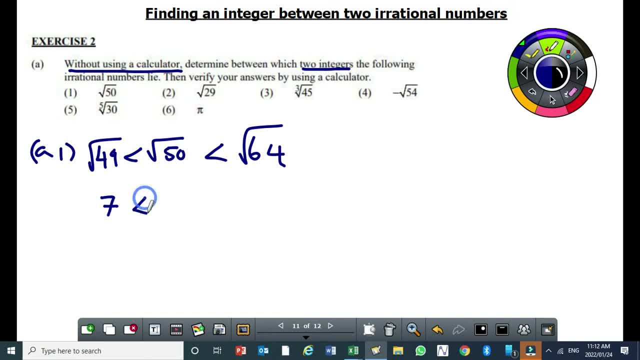 64.. But the square root of 49 is a 7.. The square root of 64 is 8.. Therefore, square root of 50 lies between 7 and 8.. 7 and 8 are the two integers, such that square root of 50 is between those two integers. 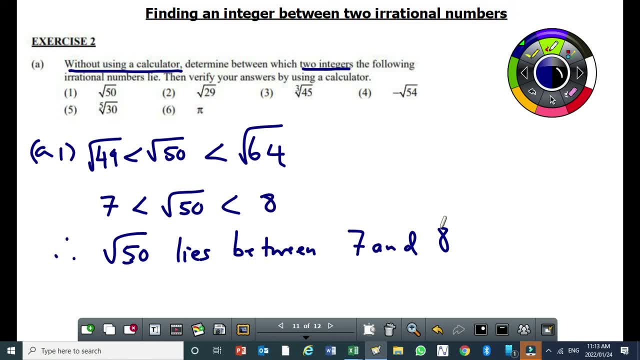 Are you following that? Yes, I get the question better, But if you don't have a question, let's move on to the next one. So I'm going to move on and do one where we have got a few roots, That's the cube root of 45, okay. 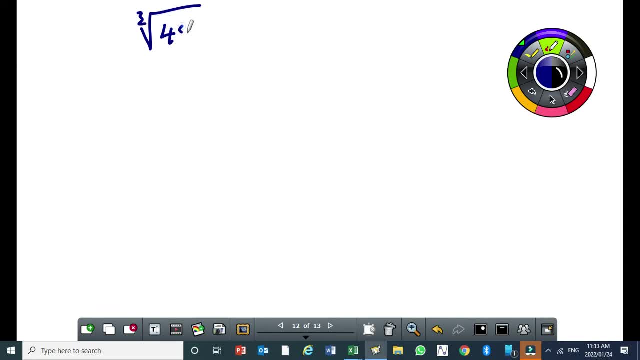 So the cube root of 45, which perfect cube is close to 45 and is also greater than 45?? What 64. So we need to find the cube root of 64. Then which perfect cube is close to 45? 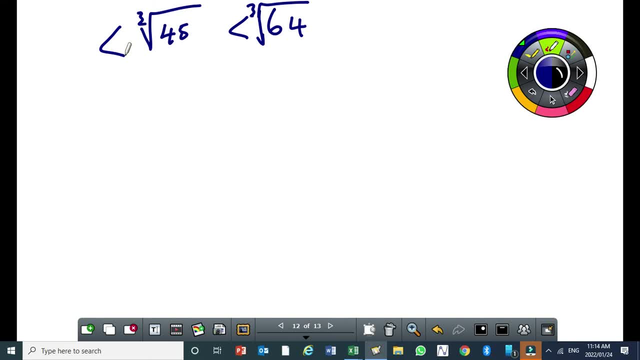 but is less than 45?. And then we say: so, this is number three there, Right? so the answer we'll get here is the three, and then we'll get the four. Then we say, therefore, the cube root of 45. 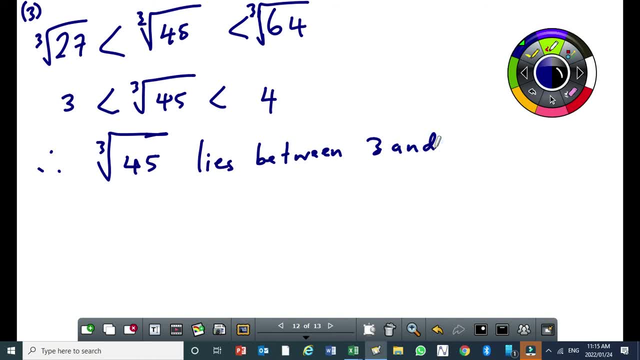 lies between three and four. Okay, Check, this is eas 막. I'll give you homework That I'm going to do. let me show you why. we'll just work negative number. Let's do one with a negative number, then we'll do the one in your textbook as well. 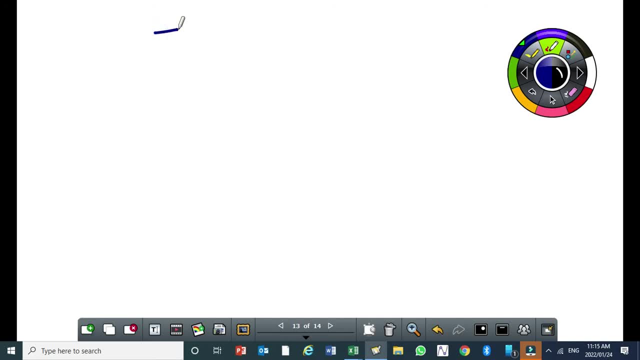 Let's say you need to find two integers that are between, say, minus the square root of 35. Now it's a negative number. This is negative: square root of what Of 35. Now, when you are dealing with one which is negative, the thinking must be slightly what Opposite. 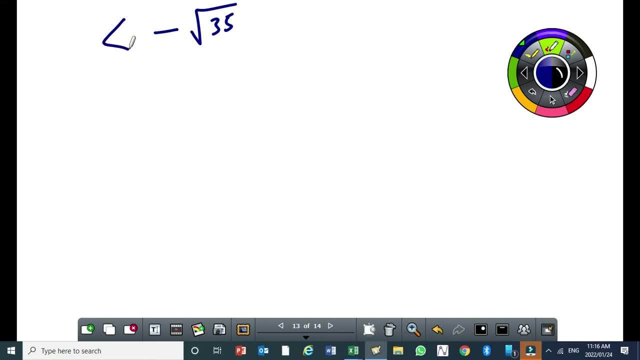 So first we need to know which perfect square such that, when it's negative, its square root, which is negative, is close to minus square root of 35.. Let's start with it as a positive. Which perfect square is positive and is very close to 35??